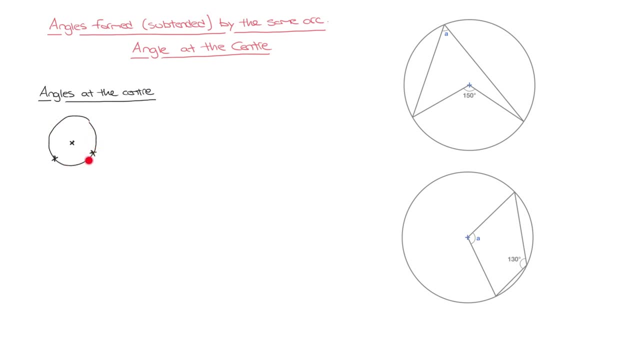 and another one could be here. I can think of the circumference of this circle as being split into two arcs. One of the arcs is this part of the circumference, That's this short arc right here, And the other arc would be this part of the circumference That's the longest of the two. 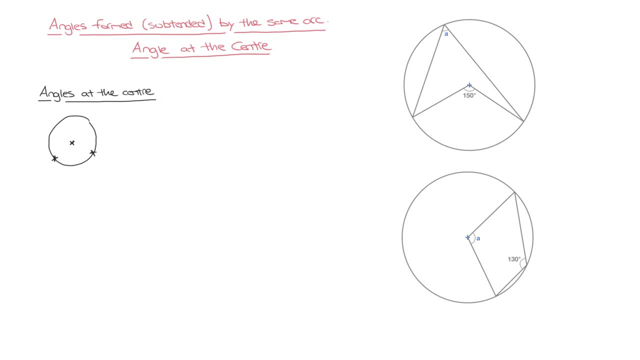 And now, if I join these two points to the center of the circle, if I draw a radius here and another one here, then that creates two angles at the center And we say that each of those angles is subtended or formed by one of these two arcs. This angle at the center. 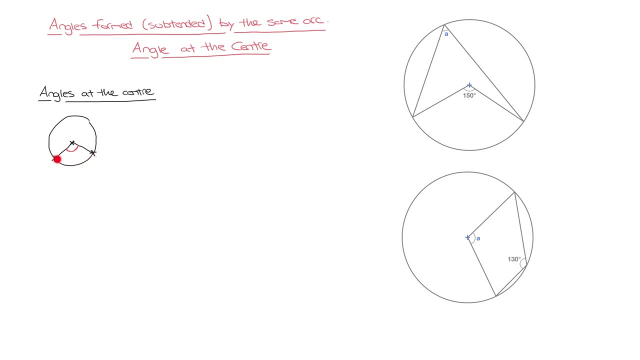 is formed by this arc here, which we can see here is the shortest of the two arcs And in fact I'll draw over it in red as well. There we go. So this red angle is subtended by this red arc. The second: 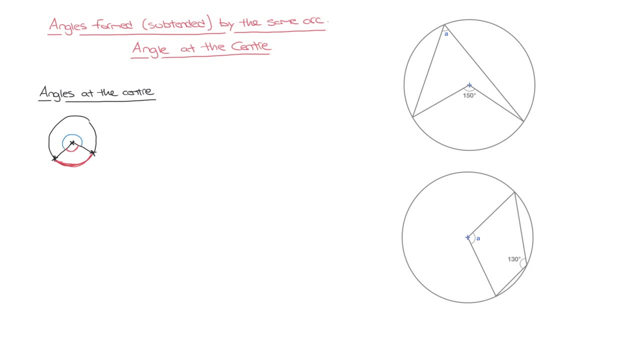 angle at the center is this angle right here, And that angle is subtended by this longer arc right here, And, to be consistent, I'll draw over that in blue. There we go. Okay, so those are the two different types of angles that can be subtended or formed by arcs at the center. But what about? 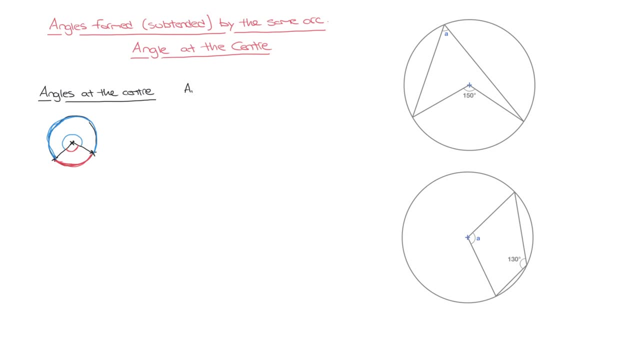 angles at the circumference, And that's the second thing I want to talk about before we actually look at the rule: Angles at the circumference. To picture things well, this time I'll draw two circles, So that's one, and its center would be right here, And in fact I'll just copy that. 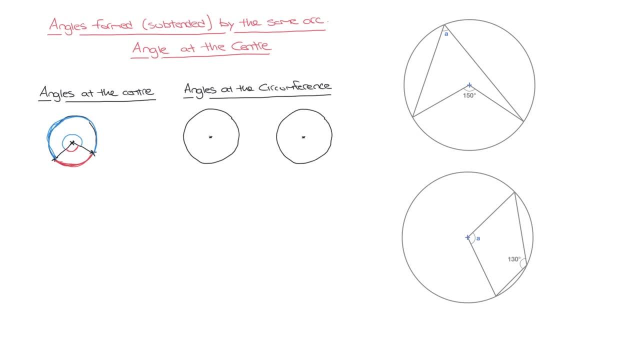 There we go, There we go. That's another one. Okay, now, once again, my starting point is two points at the circumference of the circle, So I'll play- There's one there and one there- And just as it did here, placing these two points at the 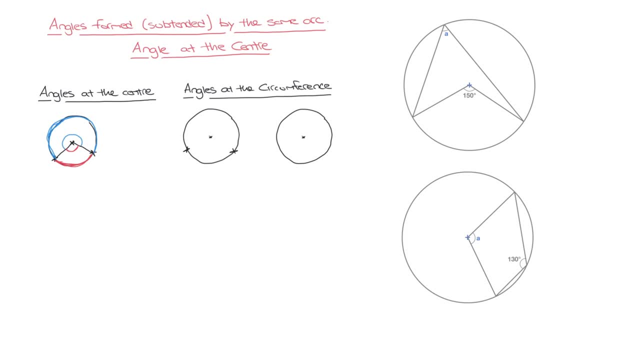 circumference of this circle creates two arcs: A short arc here and a longer arc right here. But now to picture angles at the circumference. I'm now going to place a third point along the circumference of this circle, And for this first one, I'll place that point on the longest of the. 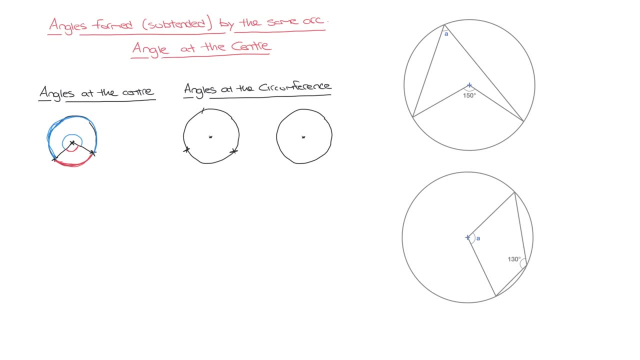 two arcs, And it could be anywhere on that arc, but I'll place it right here Now. by joining that third point to the two points I had previously placed at the circumference, it creates what we call an angle at the circumference. And that would be this angle right here. And once more we say that this angle 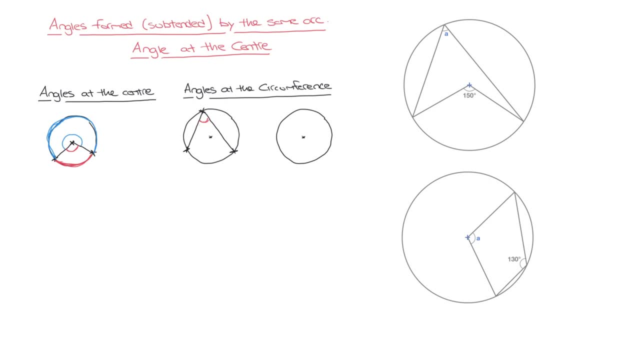 is subtended or formed by an arc, And the arc that's forming this angle would be this arc at the bottom here, the shortest of the two arcs, And in fact I'll draw over that arc in red like so. And it's worth pointing out that by placing my third point on the longest of the 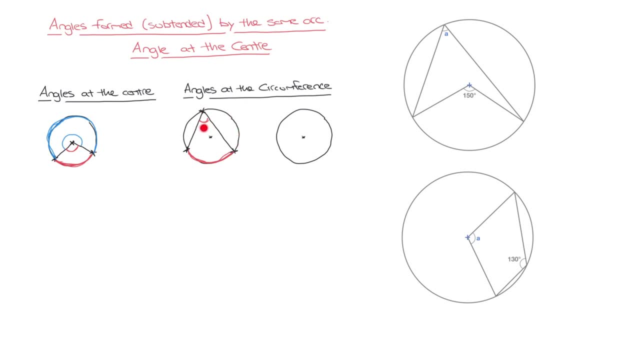 two arcs I started off with. it created an angle at the circumference which is formed or subtended by the shortest of the two arcs, And the opposite would have happened if I had placed the third point on the shortest of the two arcs. And so let me illustrate that with this second circle. 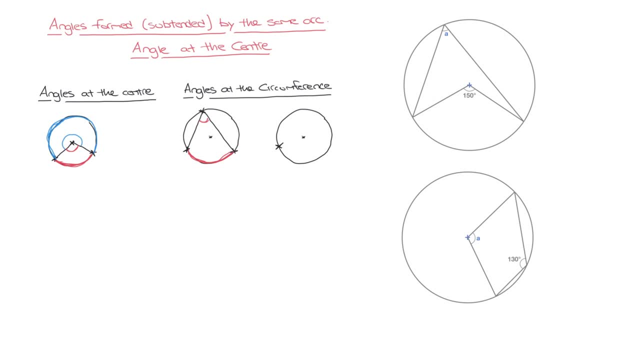 And I'll set things out the same way again. I'll place two points at the circumference of this circle, like so, And it therefore creates two arcs: this long arc up here and this short arc down here. And now I'll place my third point along the circumference of this circle, like so, And it: 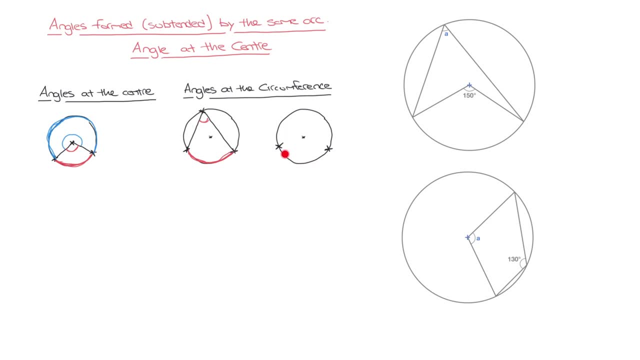 therefore creates two arcs: this long arc up here and this short arc down here and this short arc down here. And I'll place my third point along the shortest of the two arcs, so anywhere along this arc here, And I'll place it right here, And just as I did for this first circle. 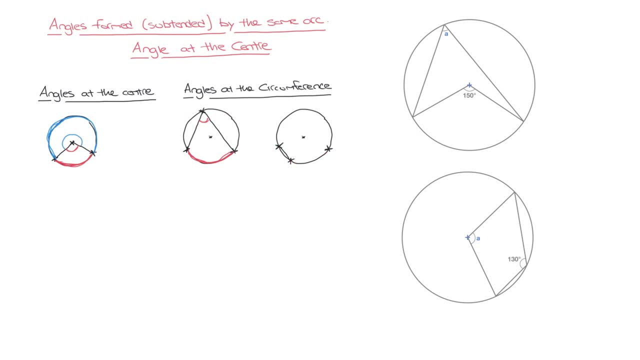 I'll join these three points, like so. And now we can see that by joining these three points, I've created an angle at the circumference. That's this angle right here, And we say that this angle is subtended or formed by this arc, which is the longest of the two, And I'll draw 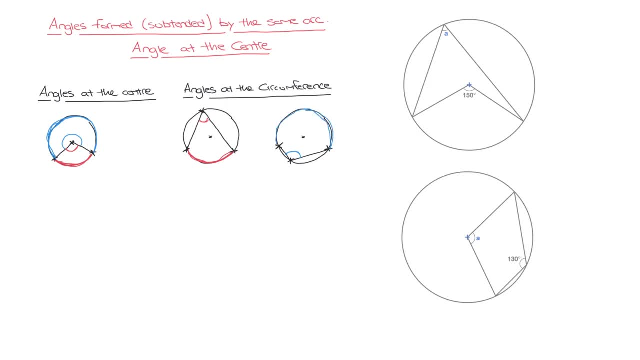 that arc in blue, That's this arc right here, And so notice that, in this case, by placing my third point on the shortest of the two arcs, it creates an angle at the circumference which is subtended by the longest of the two arcs, And it's also worth pointing out that angles at the 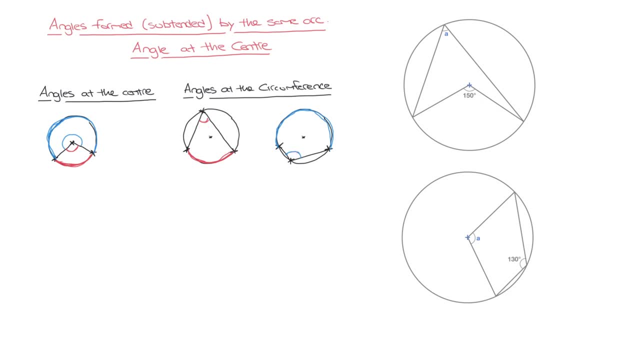 circumference of a circle can either be acute or obtuse. If the angle at the circumference is an acute angle, then it's being subtended by the shortest of the two arcs. On the other hand, if the angle is an obtuse angle, then it's being subtended or formed by the longest of the two arcs. 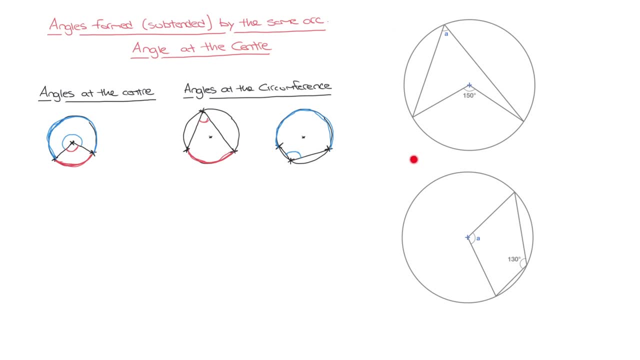 And it's worth keeping that in mind, because to answer questions like we have on the right-hand side here, the fundamental step is to figure out which arc is subtending the angles, And one of the ways to figure that out is by focusing on the angle at the circumference. So remember, if the 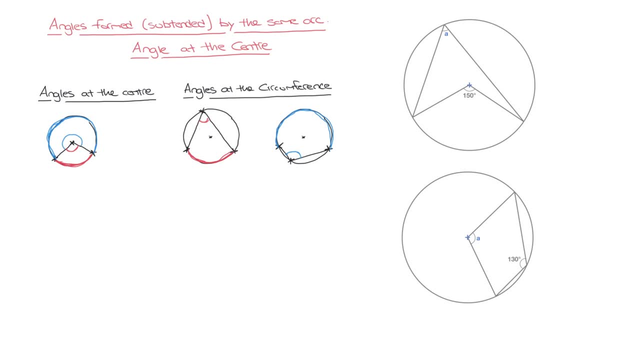 angle at the circumference is an acute angle, then it's being formed by the shortest of the two arcs. On the other hand, if it's obtuse, it's being formed or subtended by the longest of the two arcs. Okay, hopefully it's now safe to say that we know about angles at the center and angles. 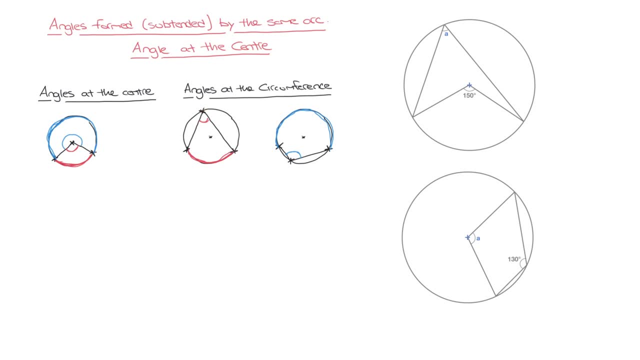 at the circumference, and we're comfortable in recognizing which arc subtends them. So let's learn the theorem, And in fact I'll go ahead and write theorem here, Just as I did for the angles at the circumference. I'm going to draw two distinct circles, And so I'll draw one. 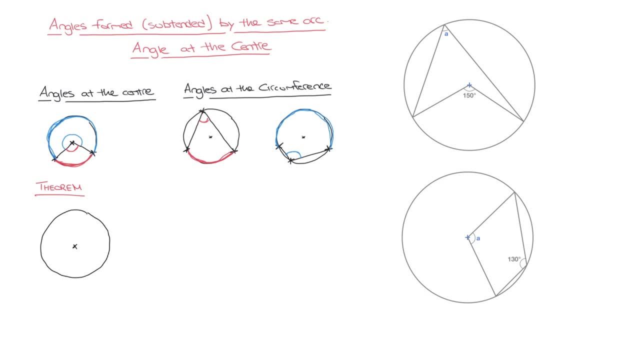 Right here And I'll say that its center is here, And I'll just copy this guy. I'll start with this circle here and I'll split the circumference into two arcs by placing two points on it, So I can place a point right here and another point right here And I'll 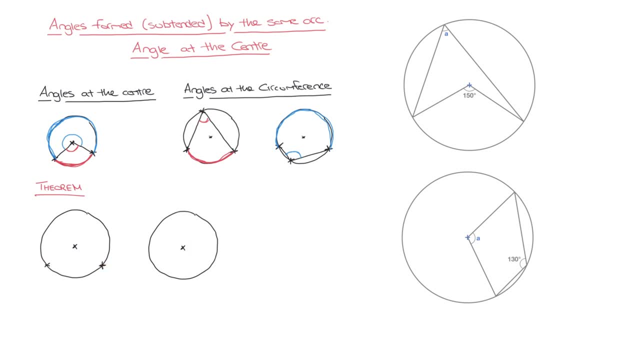 join each of these two points to the center of the circle, like so, And so we can see here that this circle's circumference is split into two arcs. We have a long arc here and a shorter arc here, And by joining the two points at the circumference to the center, I've created two. 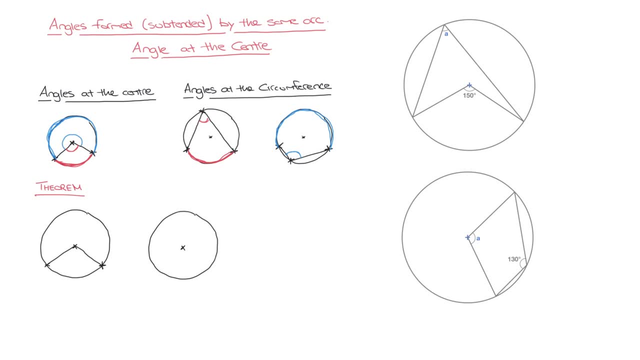 angles at the center. And so now let me add a third point on the circumference of this circle, to create an angle at the circumference. And for this first circle I'll add that third point on the longest of the two arcs, And now I could place it anywhere on this arc. 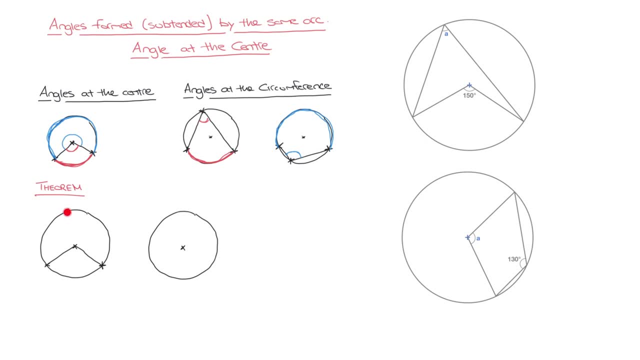 but I'll place it right here. Now I join this third point to the other two points on the circumference. So that would look like this: Okay, now what I want you to do is to focus on the angle at the circumference. So that's this angle right here. Notice that this is an acute angle. 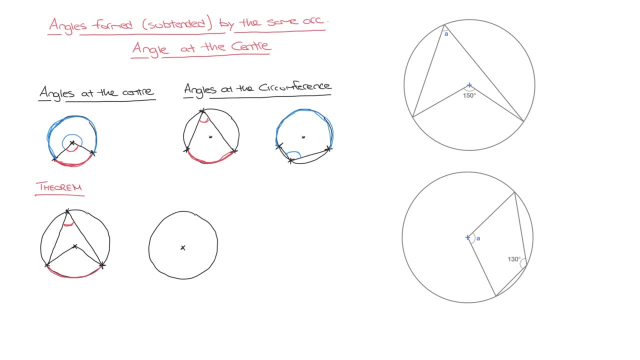 and it's being subtended by the shortest of the two arcs, this arc right here. And because this angle is being formed by this arc, this is the arc we're going to be focusing on for the angle at the center of the circle. Remember, this theorem is about angles formed by the. 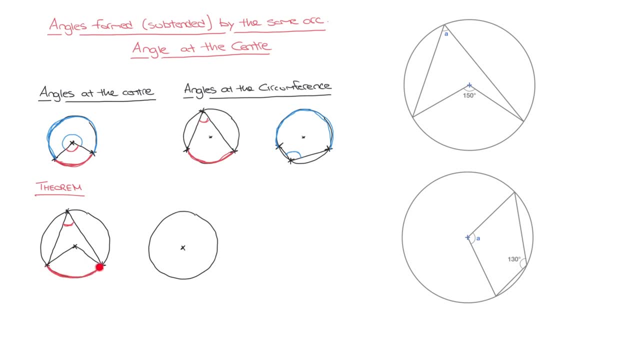 same arc, and so, once we found which arc is subtending the angle at the circumference, we need to make sure that we're considering the angle at the center, which is formed by the same arc. In other words, the angle at the center we're going to be considering here. is this angle right? 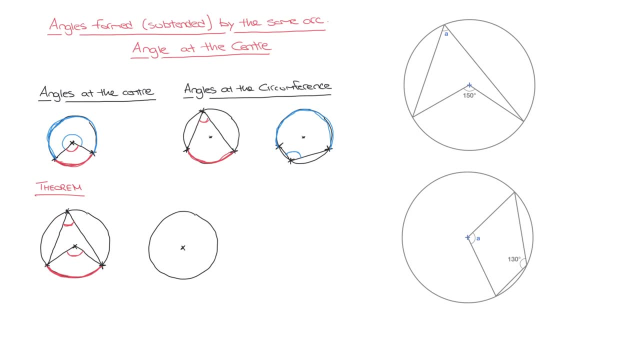 here And now. finally, what the theorem of the angle at the center tells us is that the angle at the center is two times bigger than the angle at the circumference. In other words, if I go ahead and call the angle at the circumference x, then the angle at the 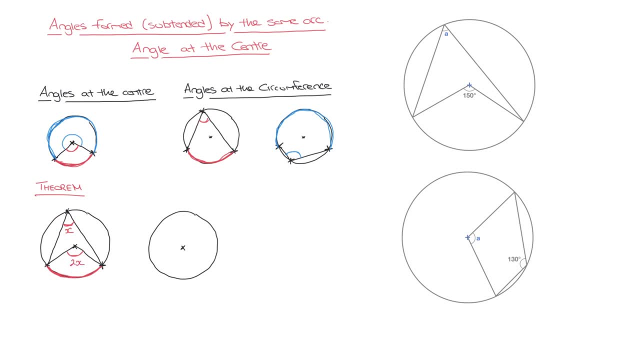 center will be 2x or 2 times x. And for the sake of being able to say that we wrote down the theorem, let me write that rule on the right-hand side here: The angle at the center is twice the angle at the circumference. 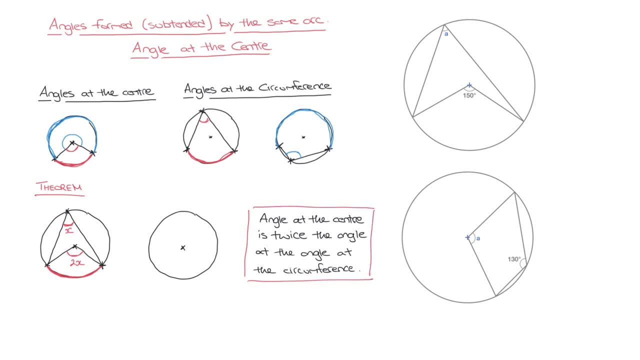 And that's the rule. Notice here that because both of these angles were subtended by the shortest of the two arcs, we end up with a quadrilateral which looks a bit like an arrowhead. But let's see what it looks like when both of the angles are subtended by the longest of the two arcs. 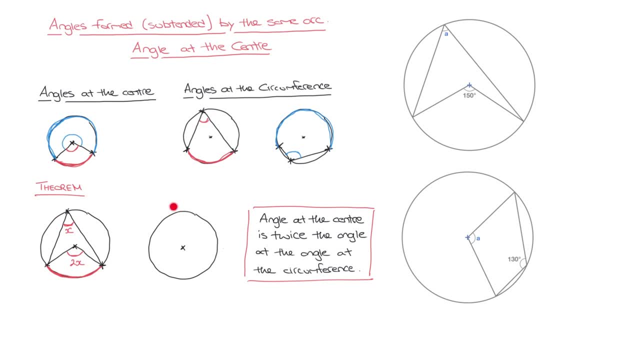 and I'll do that using the second circle. here, Once more, I'm going to split this circle's circumference into two arcs, and I do so by placing two points on its circumference, so one there and another one here, And so I now have my two arcs. I 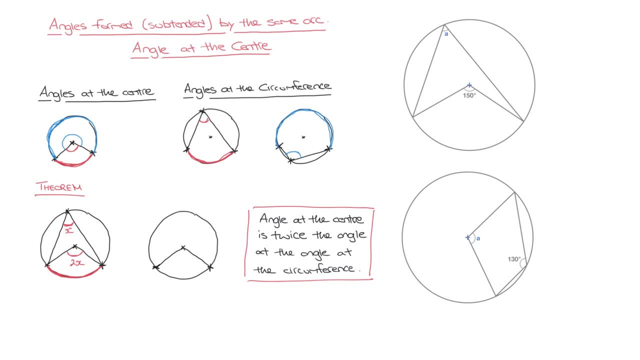 now join these two points to the center of the circle. There we go, Which again creates two angles at the center, one here and one here. And now I place my third point on the circumference of the circle, but, as I said, this time I'll place it on the shortest of the two arcs And anywhere. 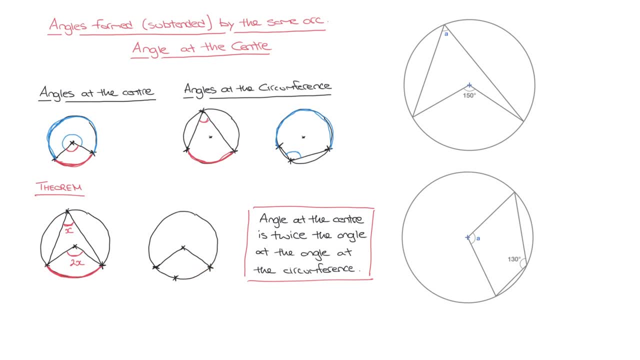 along this arc will do, but I'll go ahead and place it right here. I now join this third point to the other two points on the circumference, like so, And just as it did for the first circle I have here, joining these three points has created. 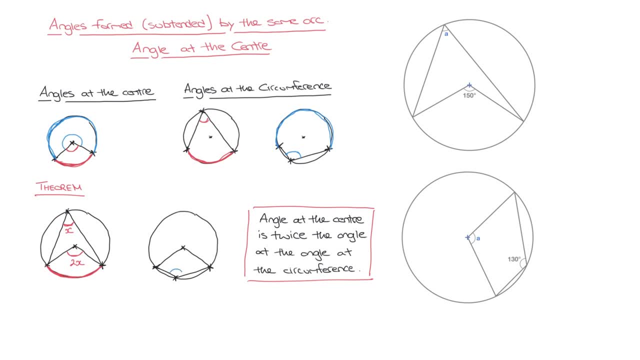 an angle at the circumference, And that's this angle right here And now the question which will allow us to figure out which angle at the center we have to work with, And that is, which arc is subtending this angle at the circumference? And I'm sure you could probably tell by 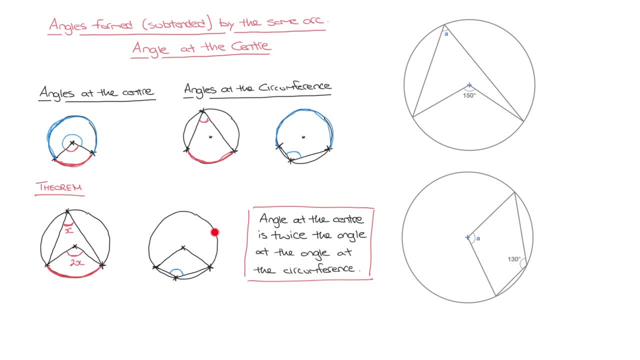 now that it's the longest of the two arcs that's forming that angle, which I'm drawing over right now in blue. And, if it helps, remember that if the angle at the circumference is obtuse, which it is here, then the arc that's subtending it is the longest of the two arcs. 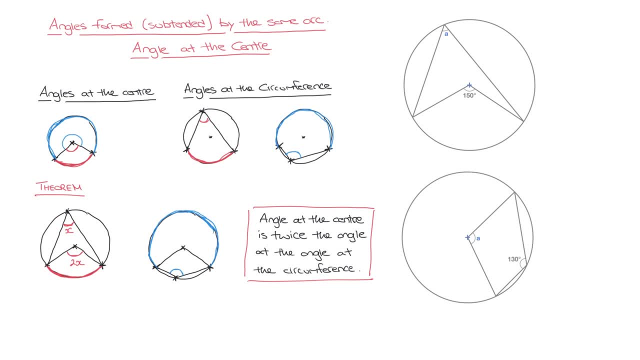 tending. it is the longest of the two arcs. Okay, now that we know which arc we're dealing with, we can quickly tell that the angle at the center we have to work with is this angle right here, And so we have an angle at the center and an angle at the circumference, which are both 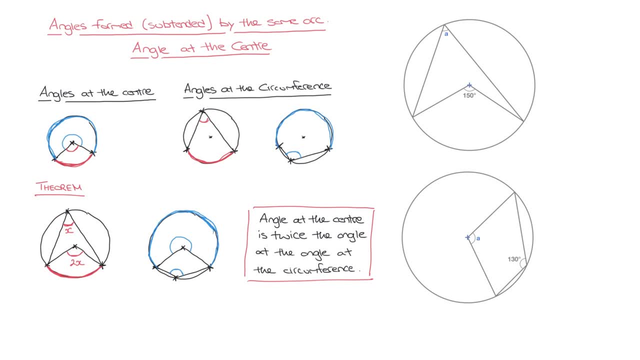 subtended or formed by the same arc and we can therefore use this rule And we can state that the angle at the center is two times bigger than the angle at the circumference. So if I call the angle at the circumference x, then the angle at the center would be two. 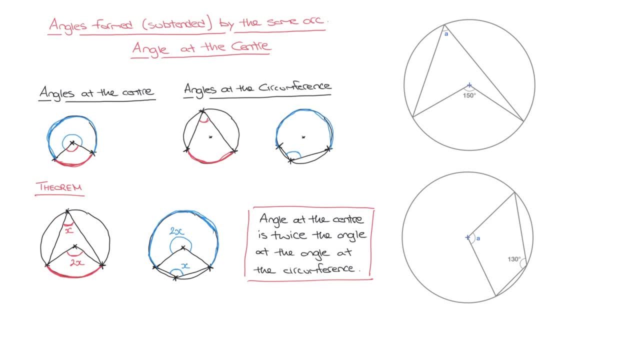 x. All right, now that we've gotten all of the theory out of the way, let's go ahead and work through these two examples. For this first example- and in fact I'll write example one here, example one we need to. 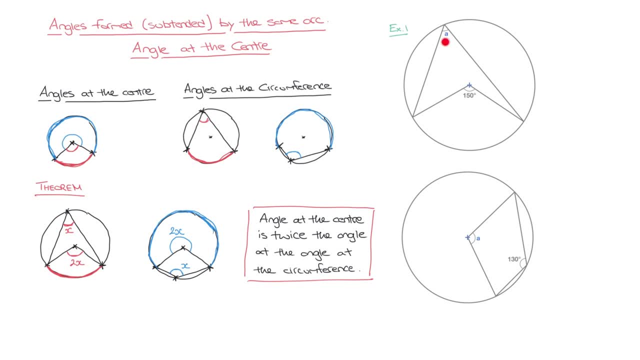 find this unknown angle a and notice that this angle is at the circumference of the circle, And notice as well that we're given an angle at the center of the circle which is 150 degrees. Now, to potentially use this theorem and find this unknown angle a, the first thing we need 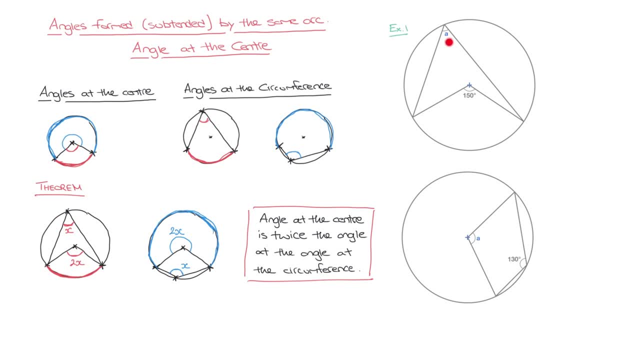 to do is ask ourselves which arc is subtending this angle. And looking at this circle, it doesn't take us too long to see that the arc that's forming this angle is the arc I'm hovering over right now, And in fact, I'll highlight it like so. 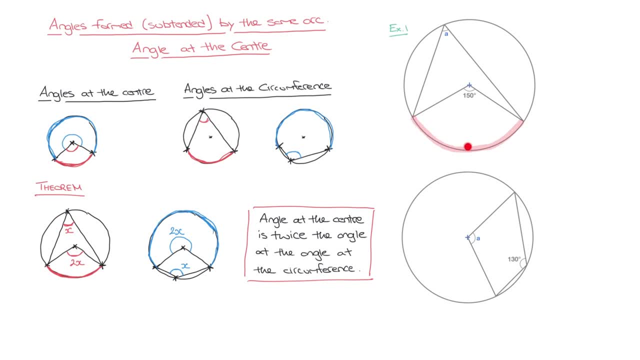 That's the arc. And now that we've located which arc subtends the angle at the circumference, We need to ask ourselves which of the two angles at the center is this arc subtending? And it doesn't take us long to see that that's this angle right here, the 150 degree angle. 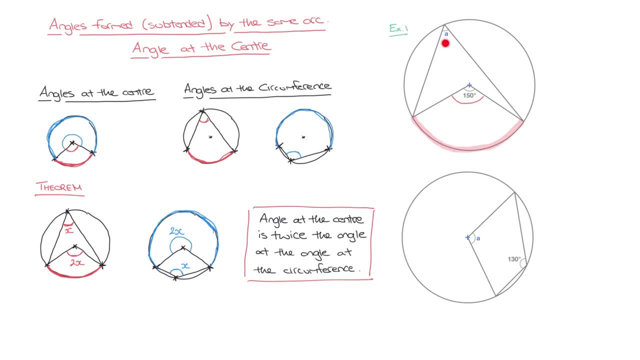 that we're given And so we can state that this angle a at the circumference and this angle of 150 degrees at the center are formed by the same arc And consequently, we can use the rule we've just learned and we can state that the angle 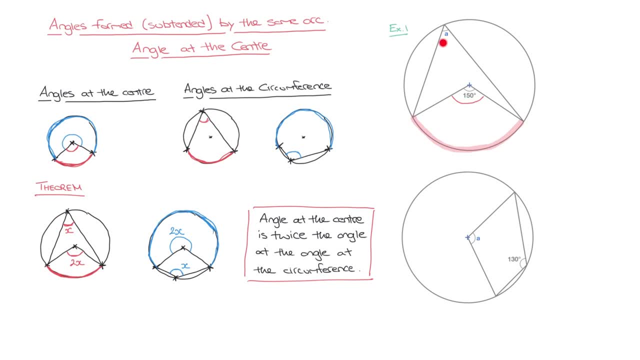 at the center is two times bigger than the angle at the center At the circumference, and we can state that 150, that's 150 degrees, is equal to two times eight. All we have to do now is solve this equation for eight. 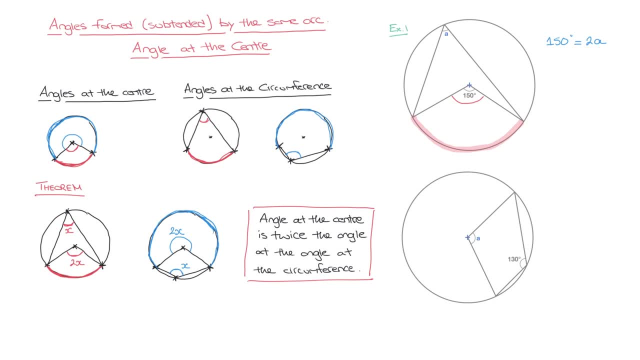 And to do that I just need to get rid of this. two, that's multiplying eight, And for that I divide both sides of this equation by two. And so on the left hand side we have 150 divided by two, which is 75, and that's 75. 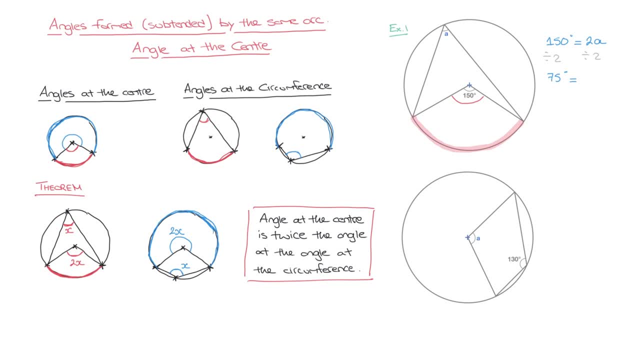 degrees, And that's equal to two A divided by two. And so we can write a equals to 75 degrees. done, Okay, let's look at the second example, And I'll just write example two here. example two, And once more we're given a circle and we need to find the unknown angle, a. 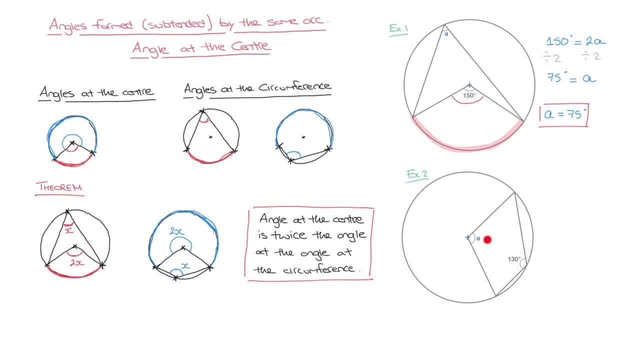 And in this case the unknown angle is one of the two angles at the center. We can also see here that we're given an angle at the circumference of the circle which is 130 degrees, And so to figure out which of the two angles at the center we can work with, we need to 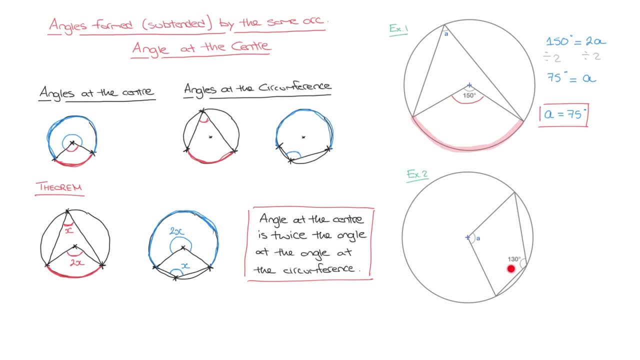 ask ourselves which arc is forming this 130 degree angle. And by now I'm sure you can tell right away that the arc that's subtending this 130 degree angle is this long arc I'm highlighting right now And, if it helps, remember, because the angle at the circumference is an obtuse angle- the 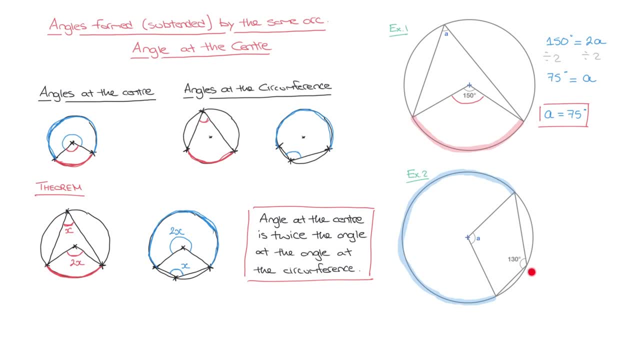 arc that forms it is the longest of the two arcs. Okay, Now that we know that we're dealing with this long arc, we can see that the angle at the center that we can use this theorem with is this angle right here, And since this angle is called a, I'll go ahead and call that angle b. 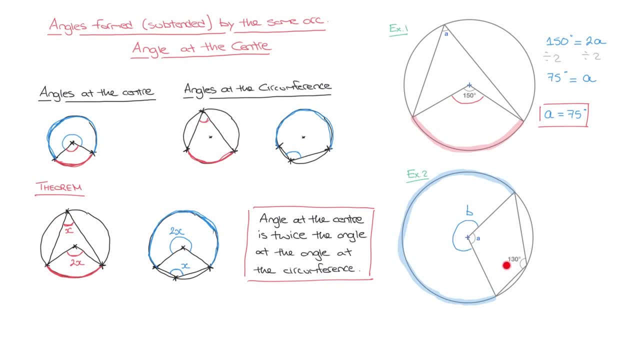 And so this angle b at the center and this 130 degree angle at the circumference are both formed by the same arc, And so we can use this rule and state that b the angle at the center is two times the circumference, Is two times bigger than the angle at the circumference. 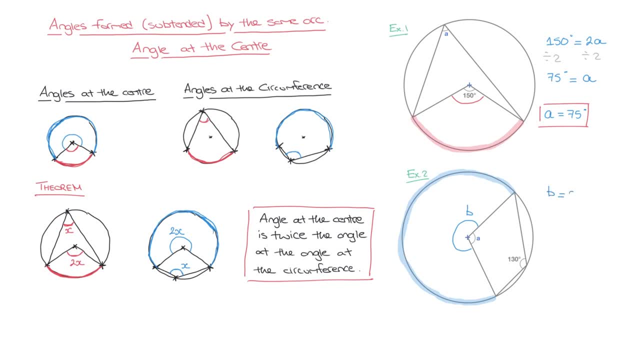 In other words, we can go ahead and write: b equals to two times 130 degrees, And so b is equal to 260 degrees. Finally, now that we know what b is, we can calculate what angle a must be by using the fact that angles around a point must add up to 360 degrees.